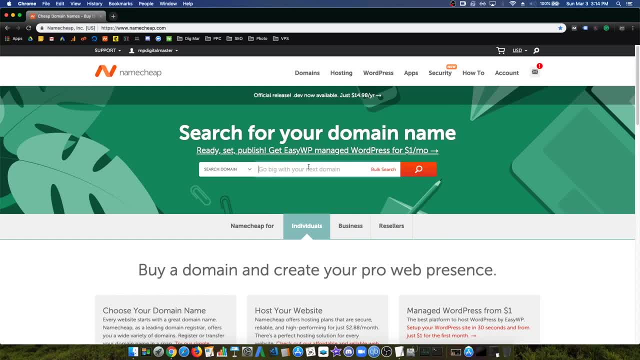 And right here in the search bar we actually get to type in the domain that we want and see if it's available. So I'm just going to choose. I'm going to choose a random domain, such as johnbrownxyz. As you can see on the top, it's actually available. 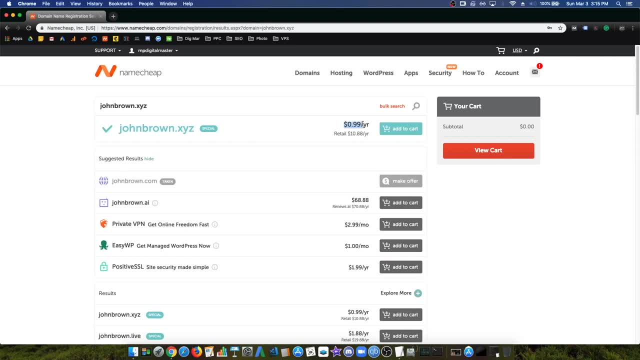 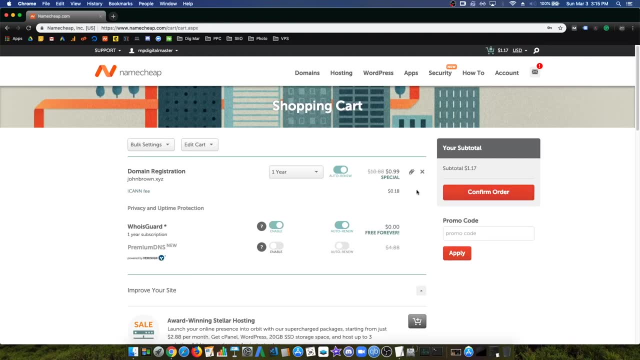 And it's going to be a purchase of basically $1 every year, So we can just add that to the cart If you view the cart, And two things. So right here. all we know this is set by default. Same thing with WhoisGuard. 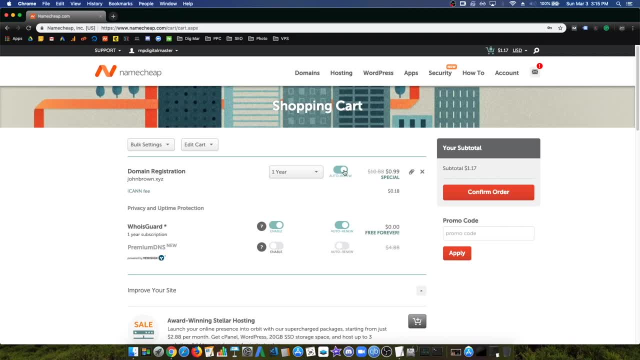 So this is going to pay every year of your domain so you can attain ownership, And it's going to collect your private information from anyone who tries to grab it, So it's going to hide your home address, phone number, anything else that's considered private. 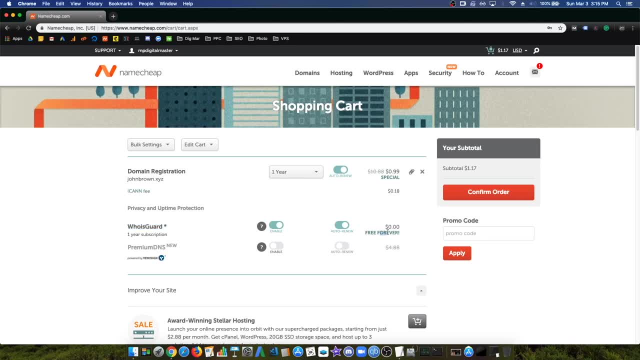 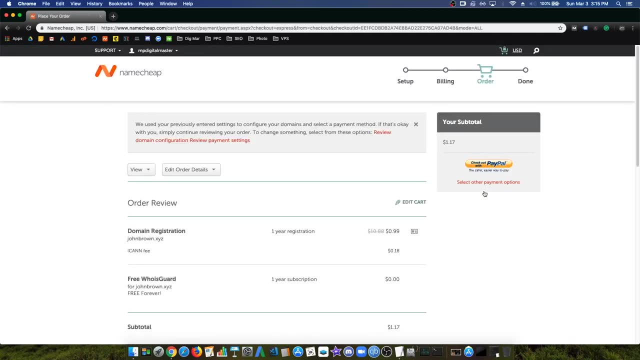 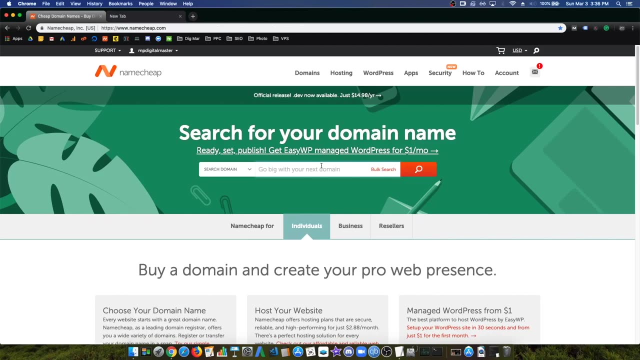 So this is enabled by default and it's free forever, So definitely have this enabled before you purchase. So, since we checked everything, so let's go over to confirm order And just use any payment method that you have, All right, So once that's done, you're going to head over to your username. 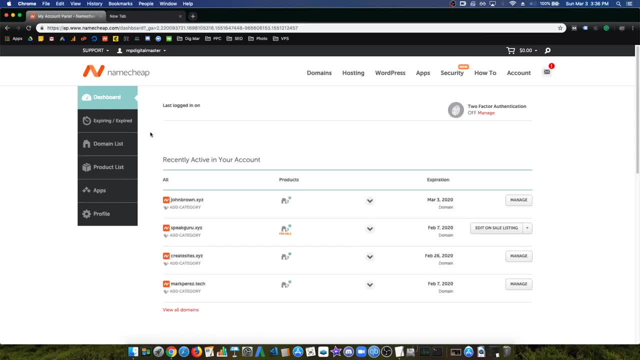 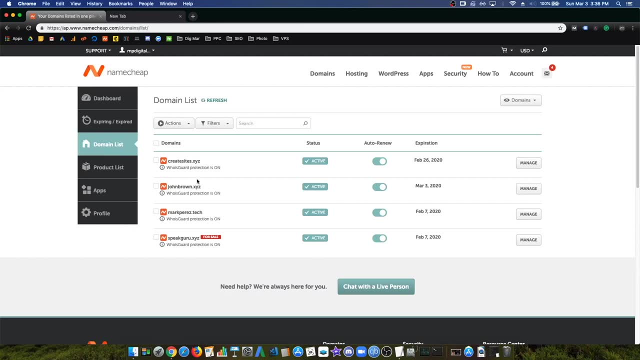 Hover over and click on dashboard, Click on domain list on the left-hand sidebar And you're going to see all your domains that you purchased. So obviously, since this is your first time, you're only going to see one. So for me, I've got John Brown. 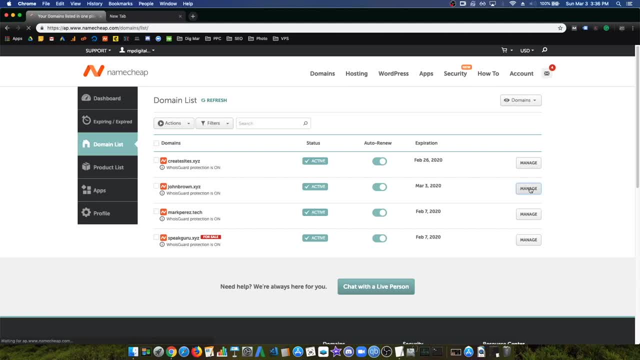 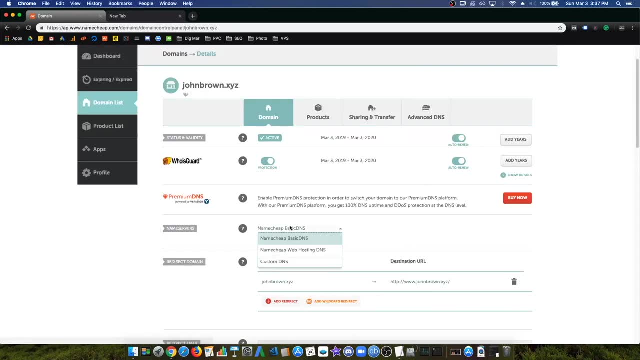 So head over to the right side and we'll just click on manage. So below this, We're going to click on name service. So we're going to be pointing to the VPS server that we want, So we're going to actually be choosing one called. let's see, it's going to be called. 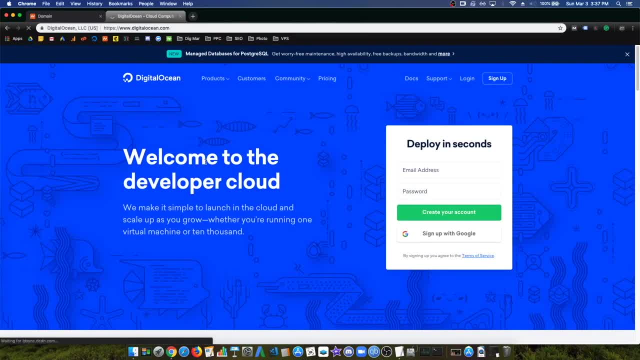 DigitalOcean. So this is going to be our service provider to host all our websites, And it may look hard at first, but it's actually really easy in the long term. So you just want to click on here and click on custom DNS. 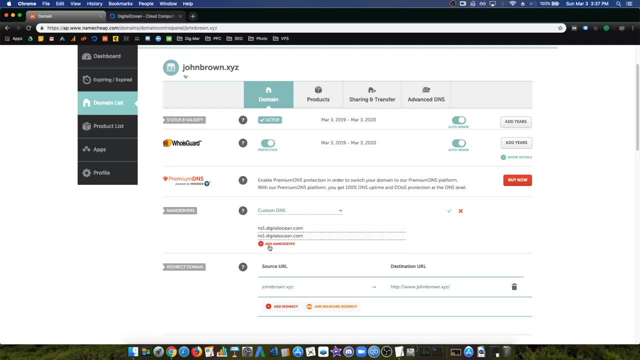 And we're just going to add this. All right, So we're going to add the name servers And again, this basically tells the domain that we're just going to. we're going to be using DigitalOcean, and then you want to click on the green checkmark. 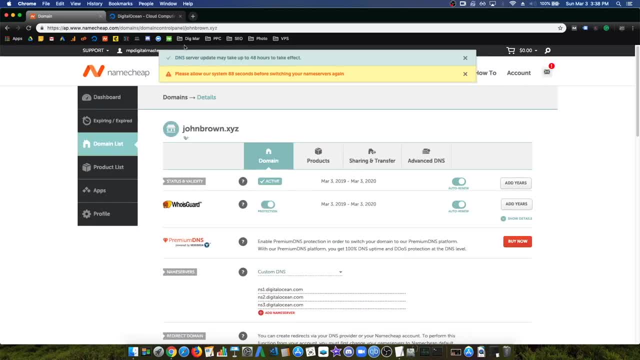 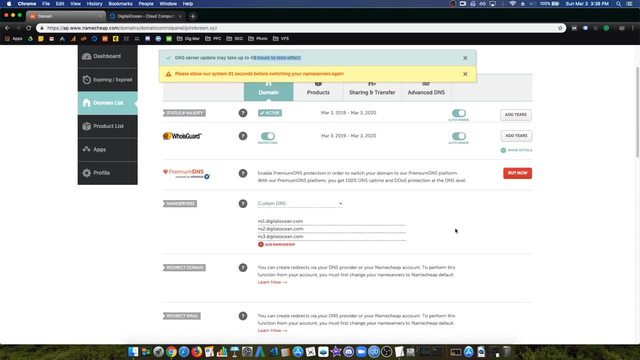 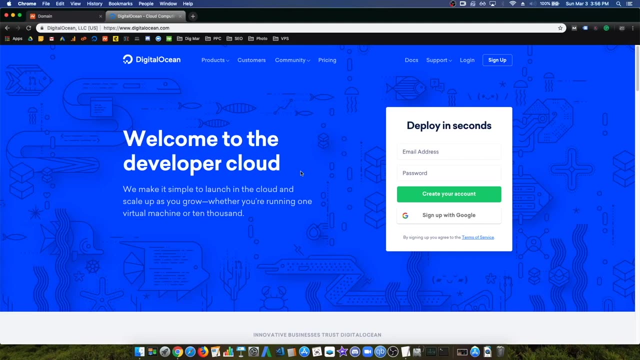 Cool, So it's set up. It does say you have to take 48 hours to take effect, but it takes around like 10 minutes, So it's not going to be too much for it to work. All right. So you want to create an account on DigitalOcean? so just go to the main web. 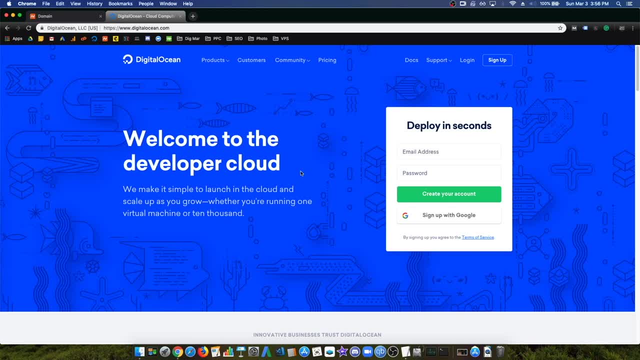 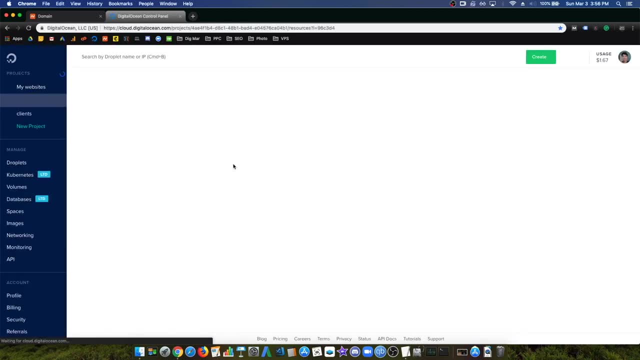 page and just sign up here and it's gonna ask you to input a payment method. so just do so and afterwards just sign in, and so here. this is basically the interface for DigitalOcean, so it might be a bit complicated for first-time users, but the only thing we're gonna care about are the projects and the 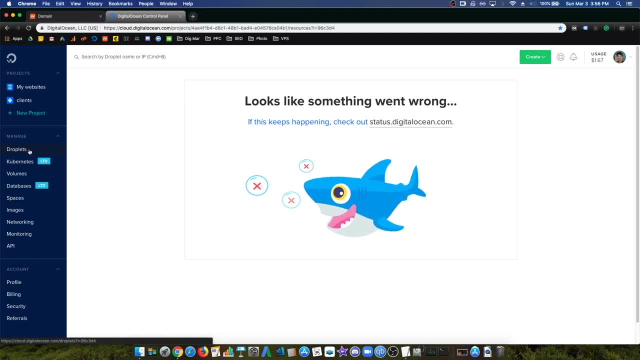 droplets, and for droplets it's basically like a. it's a code name for like VPS, but but they call it here droplets, so it's. it's basically the same thing. so the first things we need to do is a click on create a new project and 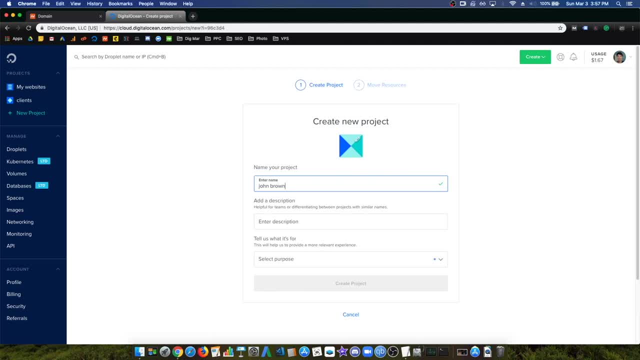 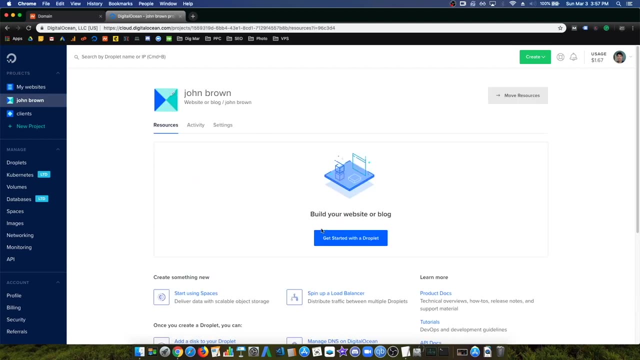 just you can name it anything you want. so I'm just typing in: John Brown, it doesn't really matter, this is just to organize your projects and just create projects and just skip for now. all right, cool, so we created our first project, so now let's create the VPS, aka the droplet. so click on the green, a green bar in the 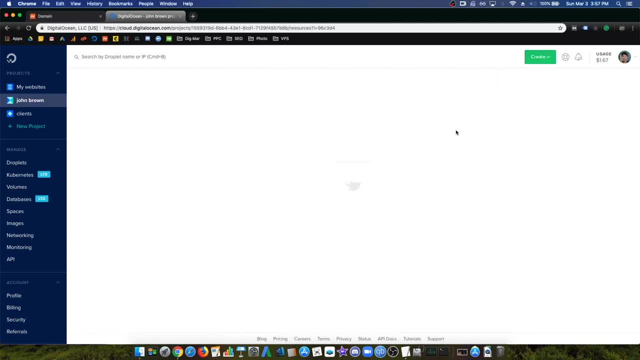 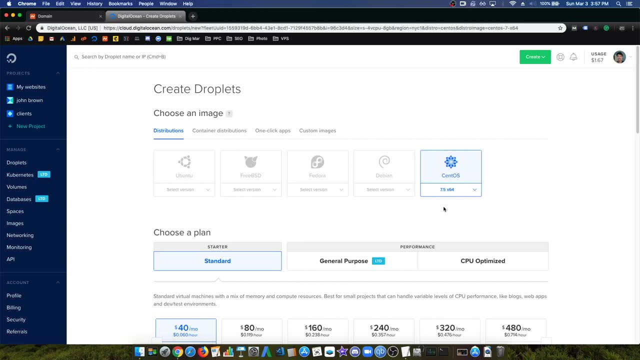 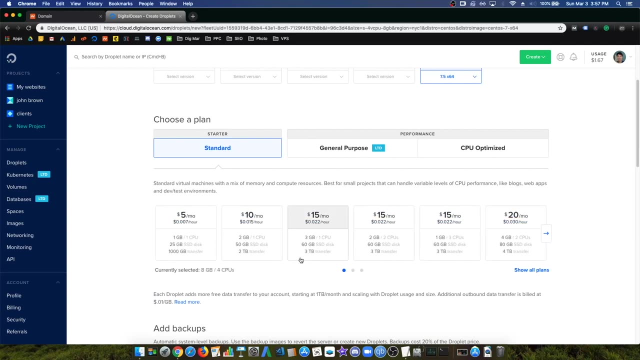 top right corner and we're gonna click on droplets. and for the operating system we're just gonna choose CentOS version 7.5 or whichever latest version you have, but for me it's 7.5 and for DigitalOcean they actually charge you on. 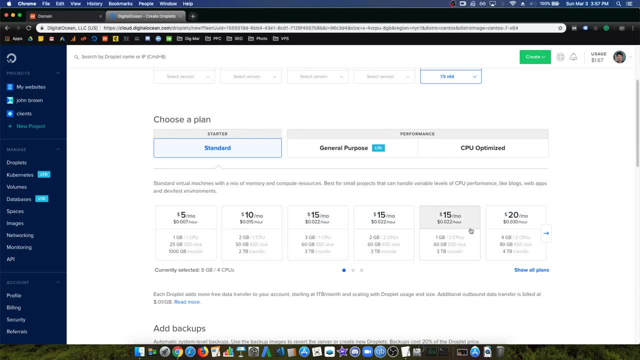 the amount of resources you actually use. so it's definitely not gonna be like 20 or 15 dollars a month. I have the $20 per month plan and actually got charged 13 dollars last month because I actually didn't really use the amount of resources I actually had available. so if you definitely use less resources and 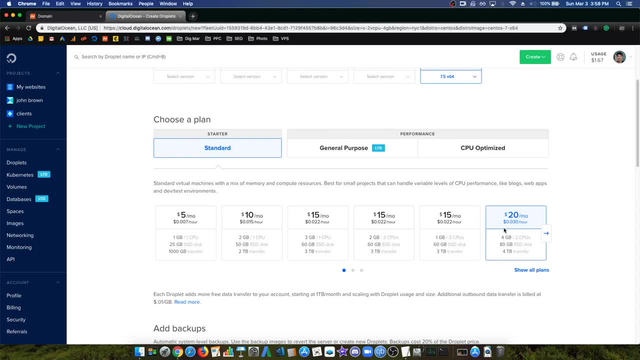 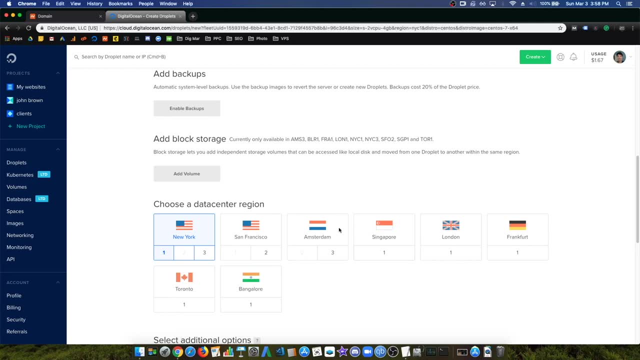 then you actually could use. you'll definitely get charged way less. so it's good, it's a good starting point to choose 20 dollars and choose the server location that you actually have located. you're, uh, mostly near, so for me i live in california, so it seems like the only option. 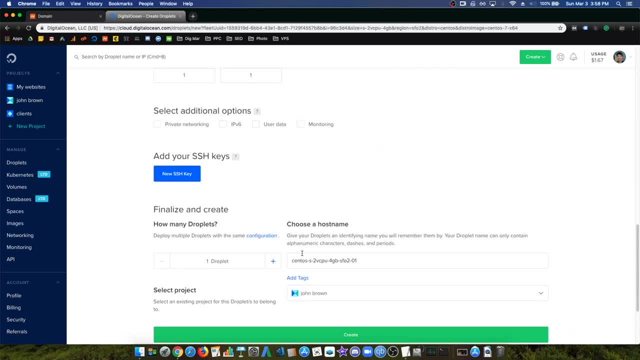 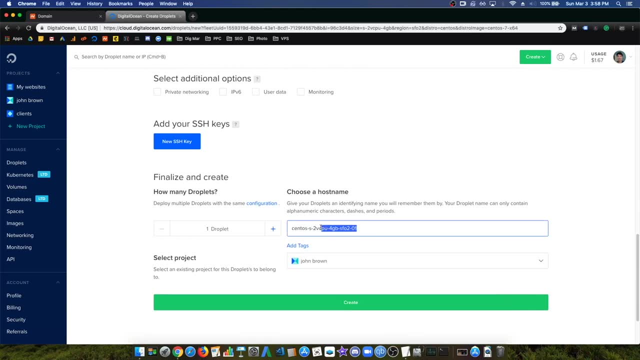 is san francisco and you'll not. you'll have to worry about the rest. uh, right here, and the only thing we care about now is the host name. so for me, i usually just call it sent west, dot your domain, john brown dot xyz. and this is actually not optional, it's actually mandatory, so it actually 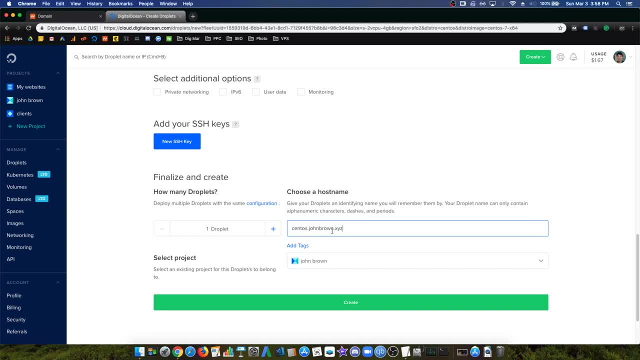 synchronizes with your domain. so, uh, so make sure you just type in: uh, whichever name you want dot your domain, uh, so this, this is the part that's actually mandatory, and for the tag is just: uh, choose your the project i created- so for me it was john brown- and just click on create. 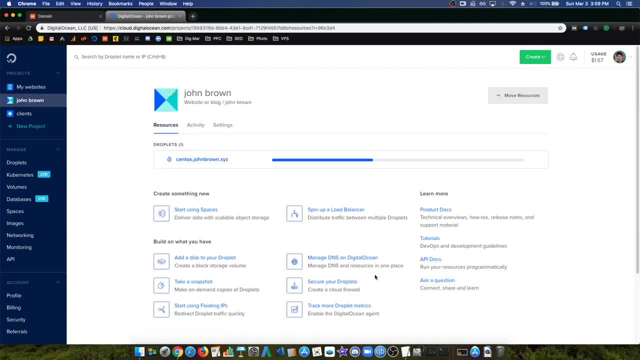 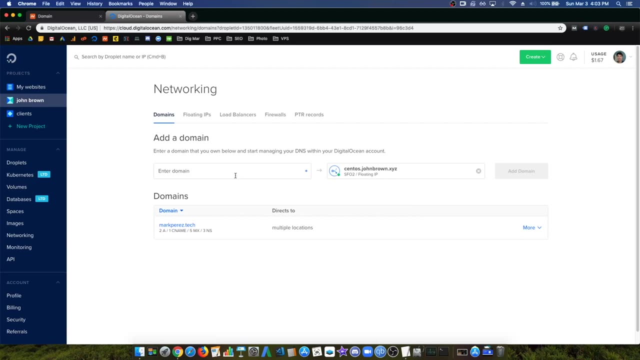 and this might take around 20, 10 to 20 seconds, so just be all right. so after the, your droplet's created. now you want to click on the red one, three dots right here, click on add domain and you want to just type in the. 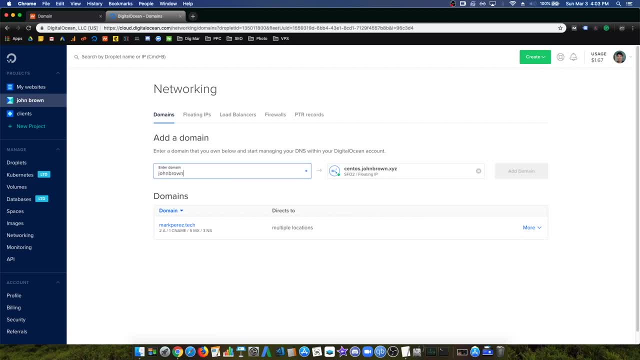 domain that you actually have. so it was John Brown dot XYZ and make sure it's a. it's actually going to be registered on your droplet with fruit, which for us it was called John Brown dot XYZ, and just add the domain. all right, so cool so. 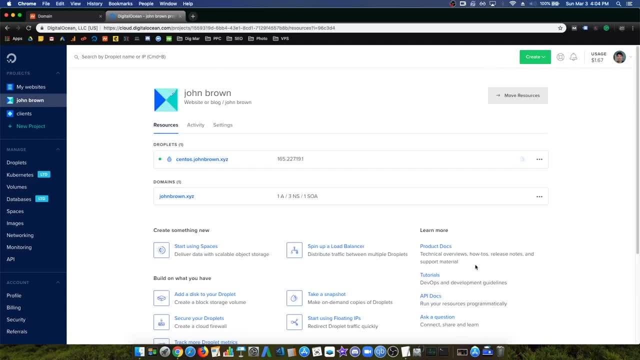 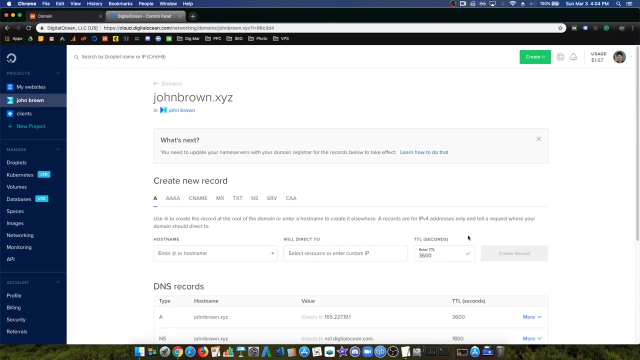 once that's done, you want to head over to the projects and click on your project and, as you can see, now it's listed on your domain. so for you just want to click on the three dots for the domain and click on manage. now, here we're gonna tweak some stuff, so 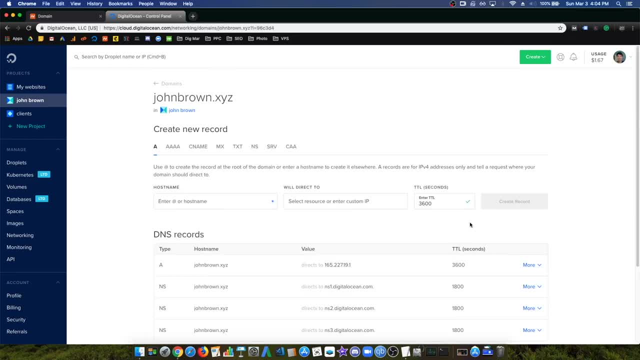 this might be a bit complicated because there's so many options. this this definitely isn't for- uh, for newcomers, but the only thing we're just gonna do is make sure that domain actually works. so when someone types in like www dot johnbrowncom, which is johnbrowncom, it will actually load the 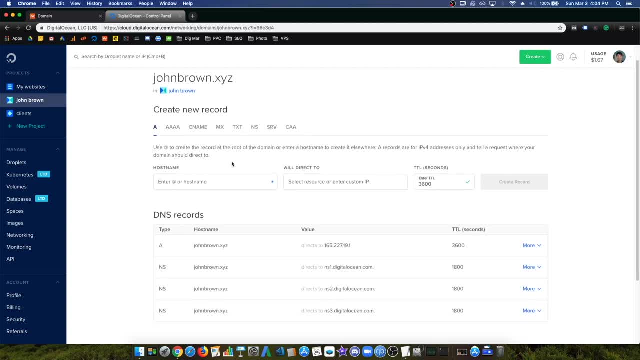 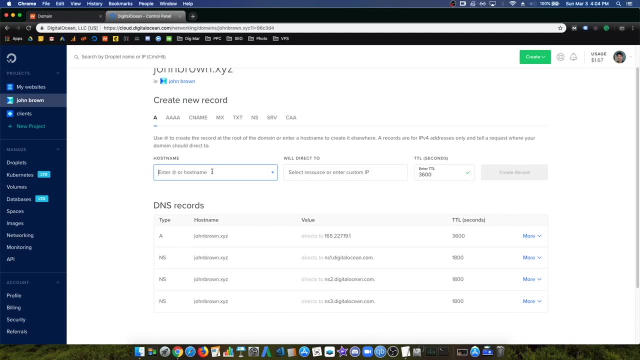 website so you're just click on a and then type in your domain. so, oh, it's actually already listed. okay, you can go back and see again, just in your domain. But yeah, just one of the useful features here is actually making sure that here. so we're just going to copy and paste. this is the domain i mean, this is the ip address for. 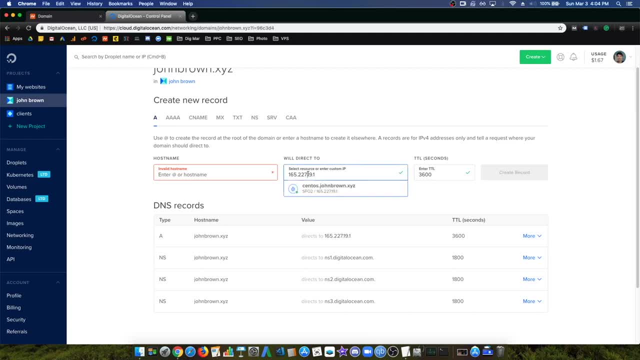 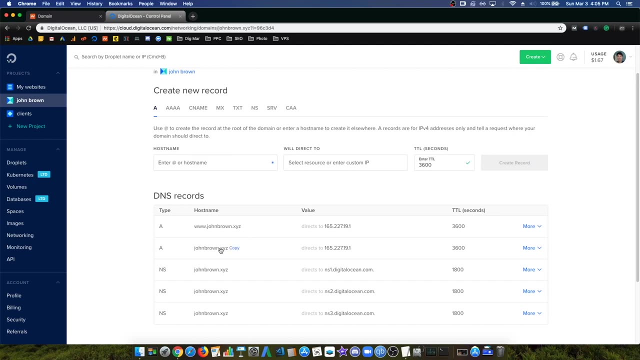 for our droplet, uh, so it's. it's, uh, we're just gonna um type in www, dot. oh, it actually already types out the dot. so all right, see, so. so for the, just the domain alone, and for the www, it's going to point for our server. so what so if the user either types in www or just the normal domain? 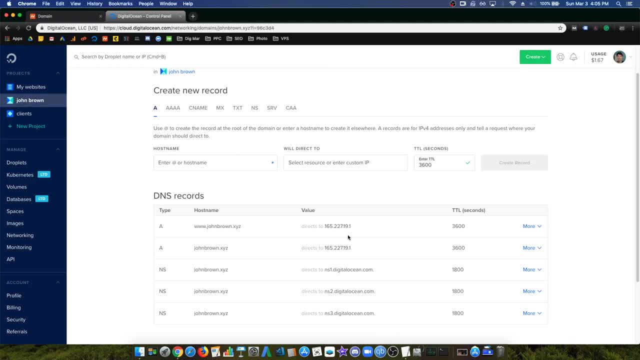 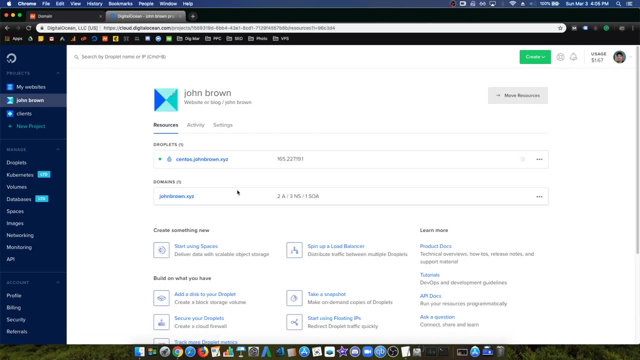 it will still work and it's going to load the website. so that's basically, uh, what we're trying to do right here. so once that's done, uh, we're all set, we can just start logging into the server and just all right. so once that's done, you're going to be receiving an email after we created the droplet. 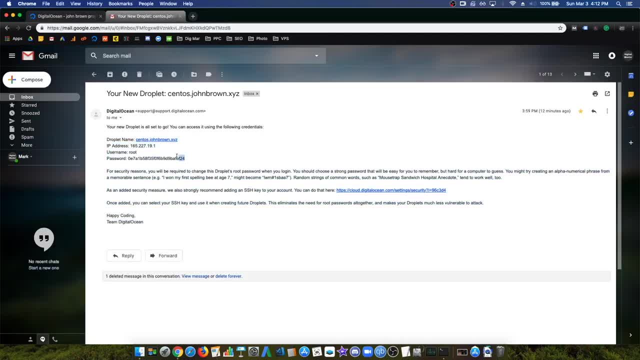 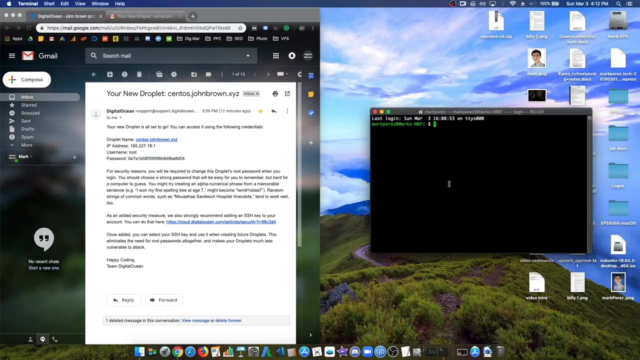 so just check your inbox and it should look like this: so it's going to give you the information in your server. uh, the only thing we need is ip address and the random generated password so to actually log in into our server. um, we're actually going to use a. we're going to use, um, the terminal. uh, since i'm using mac os, you might not have. 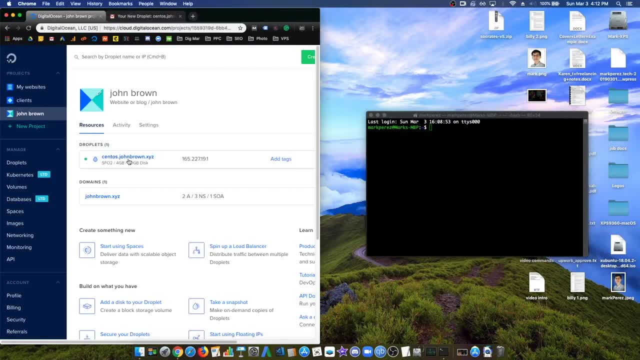 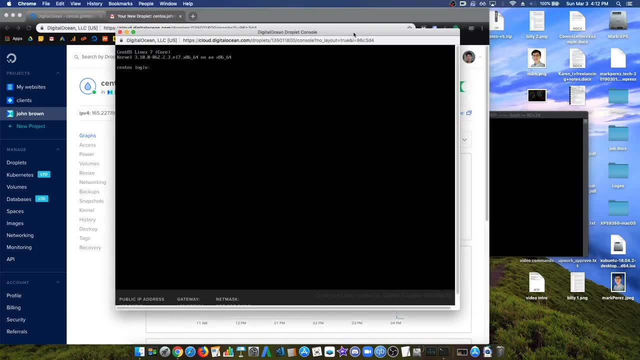 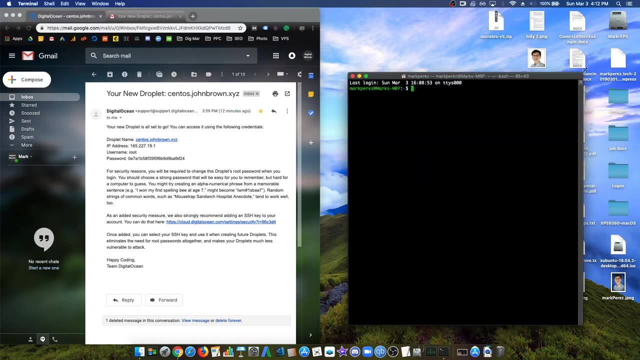 this in windows. so if you're using windows, uh, just click on your droplet and just click here, console, and for the rest of this video, just follow along using this instead. so, just, uh, head over to the email and we're gonna actually just type in: uh, ssh, uh, root at our ip. 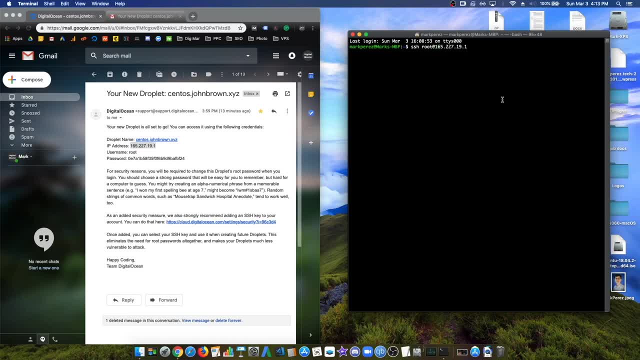 address. so make sure not to share this one with anyone, because you know they may. they might try to like log into your server. you don't really want that. you should be the only one who knows your ip address. so just try to like make this discrete, as as discrete as possible. uh, so this is the 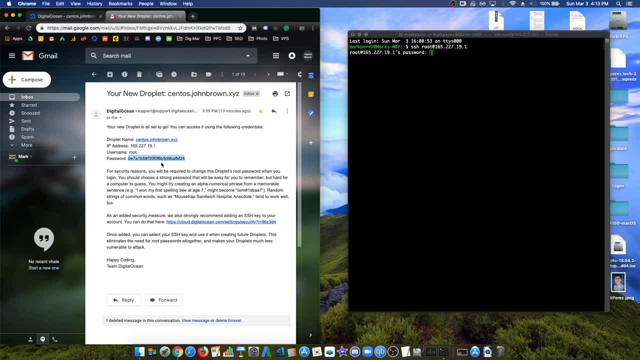 password that we actually need actually, uh turning the house, so uh just copy and paste the password from the email, uh paste it in one more time and then, right here now, you create your own password. so just create it for now. let's see that's a bit too short. 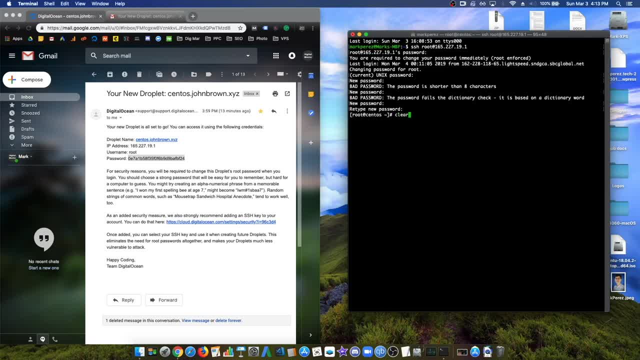 all right, cool. so now we're logged in, just type in clear. so, um, we basically just like want to update the computer and then like, install the most important stuff first. so the first thing we want to do is just uh, update. so we're just going to type in: yum. 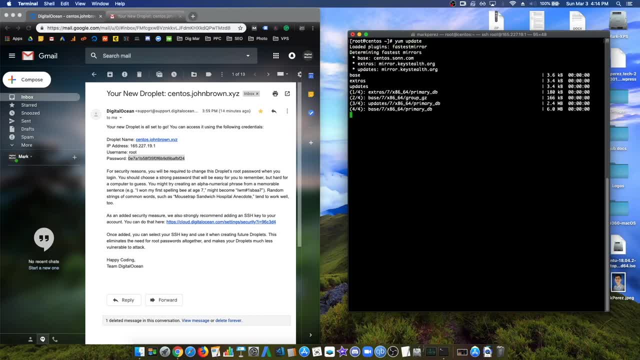 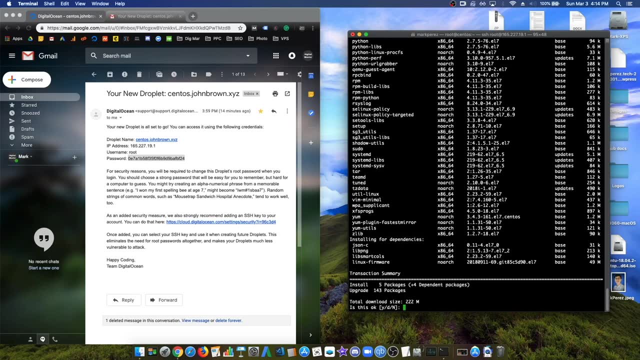 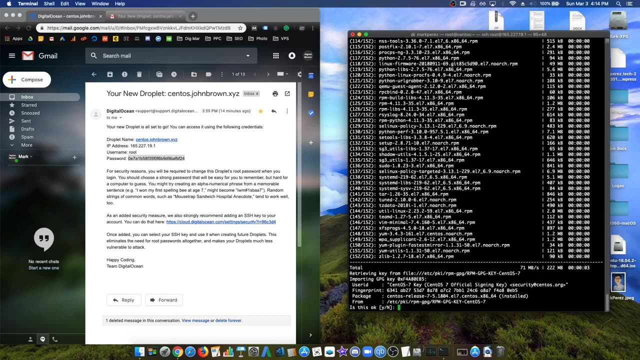 update. so it's just basically checking if there's any updates. so here's a list of updates. so all you want to just type in is, uh, type in y and then press the enter. then press enter. uh, yeah, just press enter. then download the computer, that you downloaded the computerν. 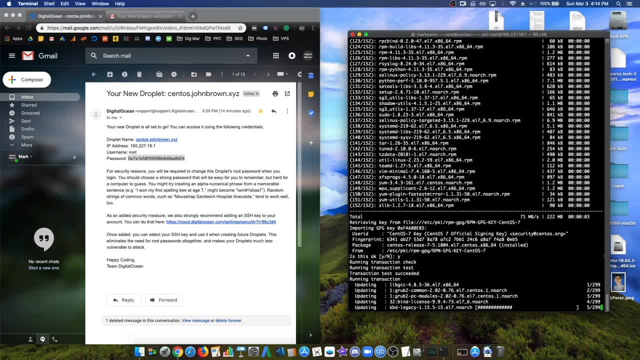 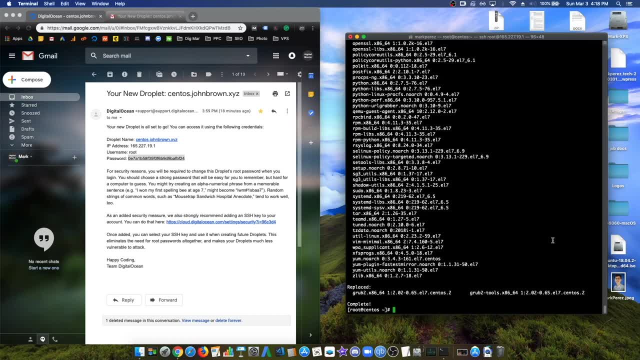 press enter, press yes and then enter for most of these. all right, so once it's finished- which you can tell because there's nothing else going on now- we basically have to restart the computer. so, um, so the updates will be applied. so all you have to do is just type in reboot, and it's just. 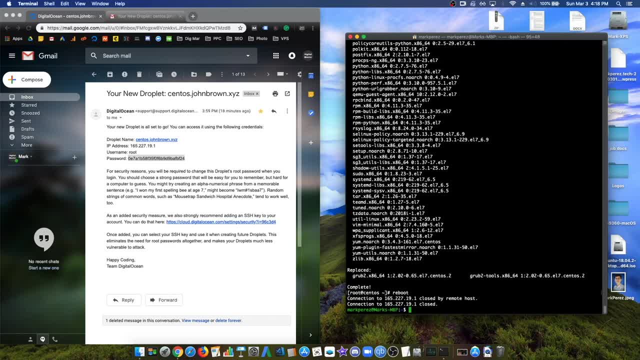 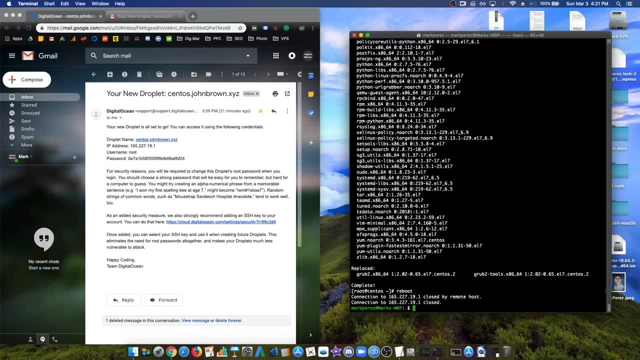 going to restart the computer and just wait like around like half a half a minute and try to re-login again. all right, so now we're going to do something pretty huge. we're going to install c panel, uh, from scratch. so c panel is basically the interface for us to configure the server. 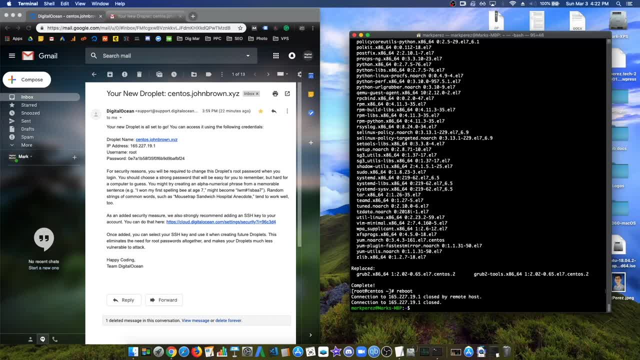 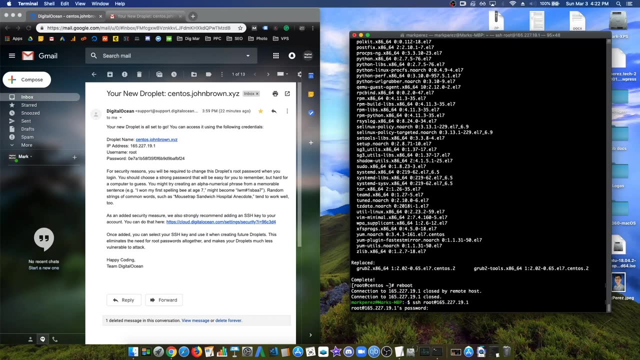 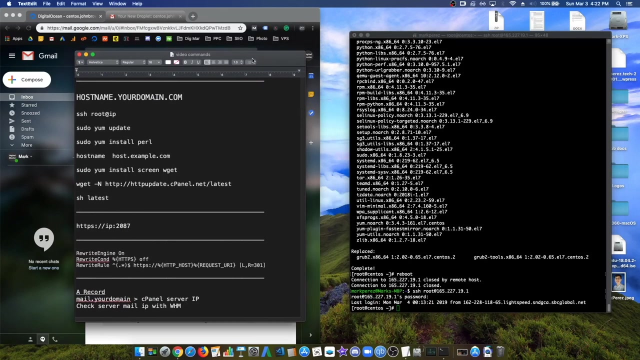 uh, like and like, configure, like multiple websites and stuff like that. so it's basically like a standardized interface for uh for anyone to use. so, um, let's just log in back to the server and type in your own password this time. all right, so cool, um, so we're going to be using some. 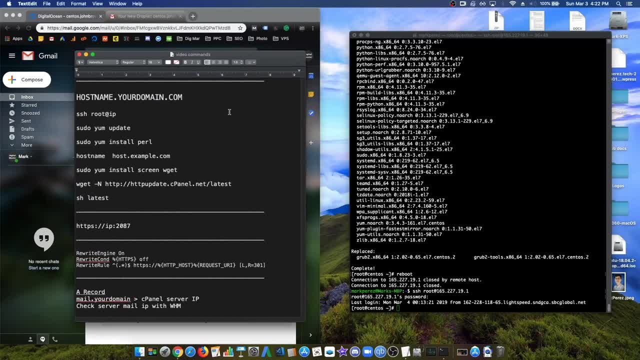 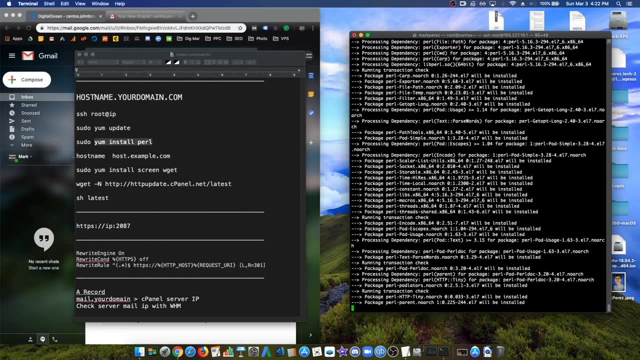 commands. so, don't worry, you only have to do this once and you can. you'll never have to like really use this terminal ever again. so, um so, uh, we already updated the computer, so now we're just going to install a programming language called pearl. uh, just press enter. oh, whoops. 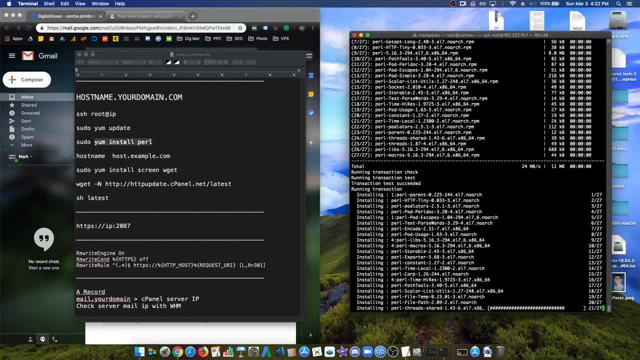 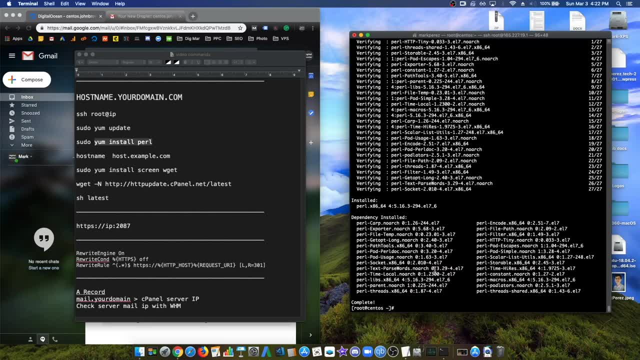 actually you have to press yes, be specific. all right, cool. so we installed pearl. now we're going to set up the name of our server. so, um, it's basically this format. so just type in host name and for us remember, uh, when we created the, it was: uh sent to us dot john brown, dot xyz. all right, cool. so we just, um, we set up the name. 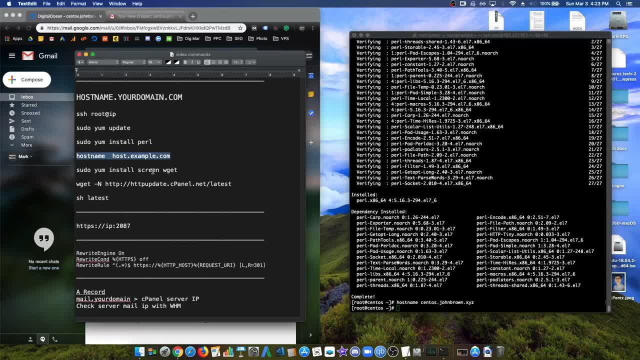 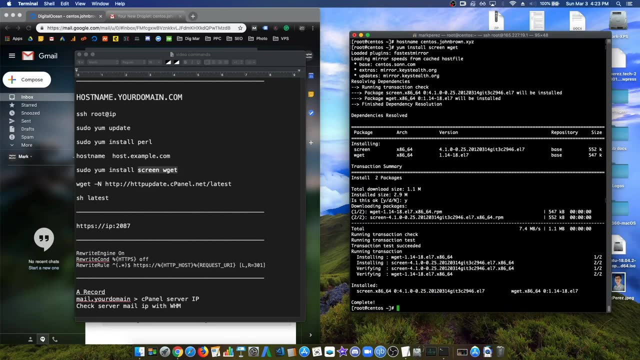 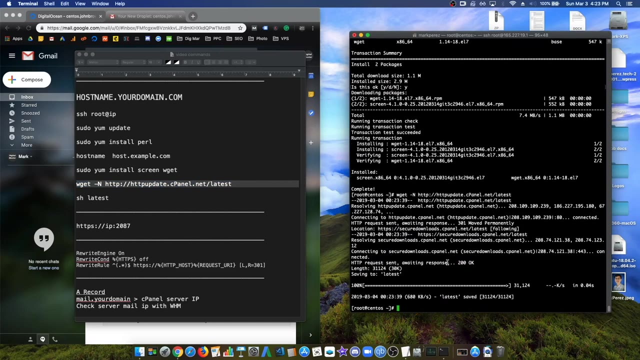 now we are going to install two programs called scream and wget. uh, install screen wget. these programs are basically going to: uh, it's going to let us download c panel, and this command right here is going to: it's going to download the entire suite, uh, so we're just going to copy and paste it. 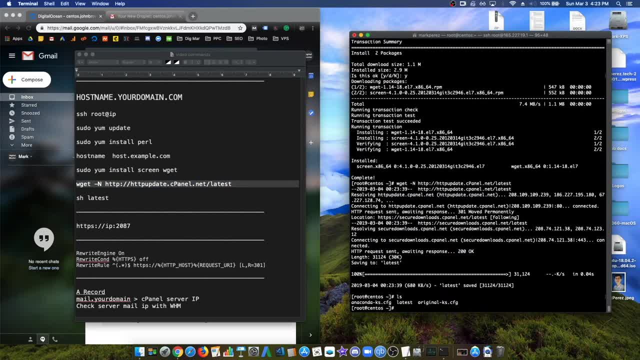 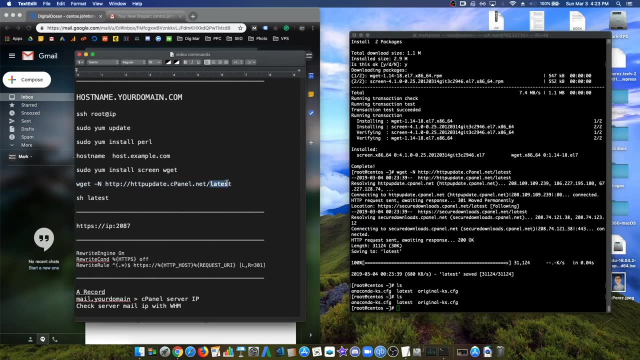 all right, cool. so um, uh. so if you type in ls- ls stands for list, uh, list, all the, all the files on on our computer. so obviously we have the latest, uh, the latest c panel uh package, which is right here, and to uh, to make it um. so with that, to make it executable, we're going to type in chum mod. 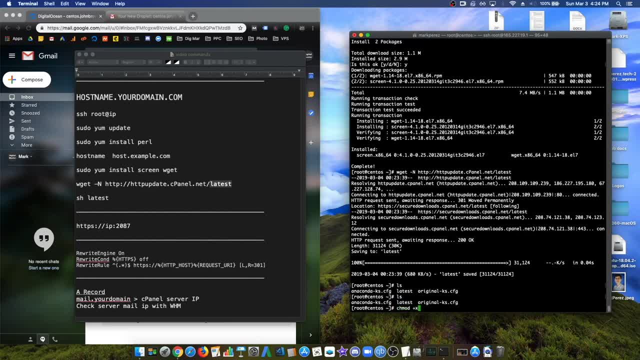 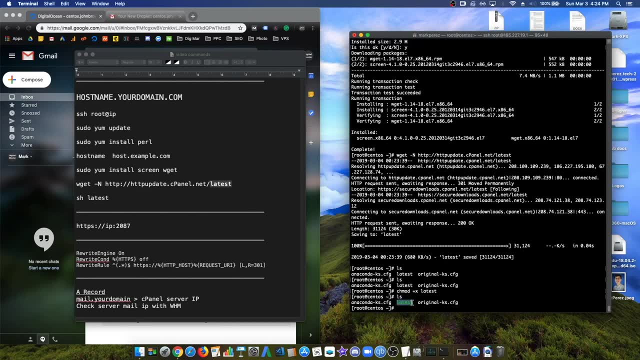 um plus x and type in latest. all right, so cool, you can see. uh, if it's highlighted green, that means that we can actually execute the program for it to install onto our computer. and now to actually run it. we're just typing, we're going to type in bash latest. i know this might be a bit different, but 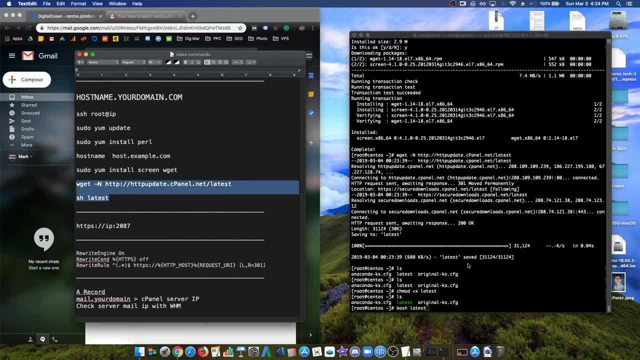 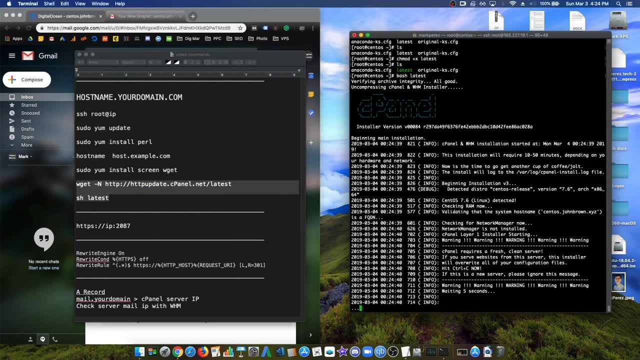 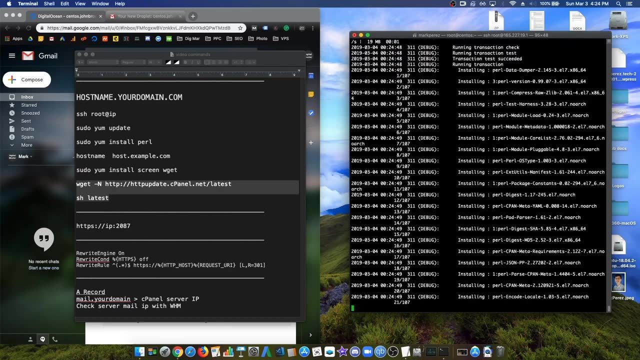 don't worry, it'll still be the same. it'll well sorry, it'll still do the same thing. so, uh, just press enter and this might take a really long time. so it depends on your computer, but i'm going to on your internet connection. this might take like an hour or two, but for me it only took around like 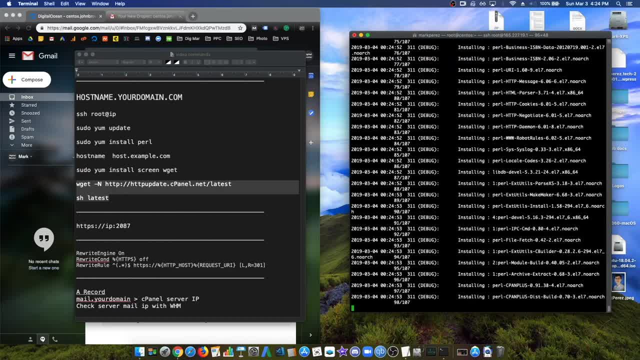 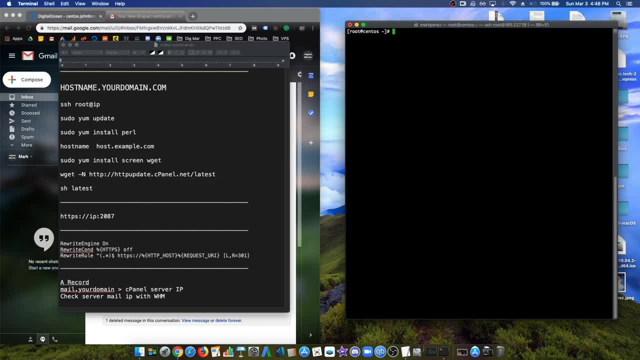 uh, like 30 minutes, so it won't take that long. all right, so once that's done, all you have to do is on head over to uh. actually, before you do that, um, you would have to just copy and paste this link, obviously for ip. you just want to type in your ip address, uh, of your server, so just copy. 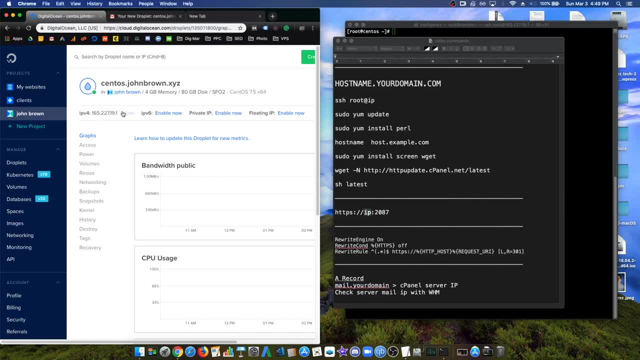 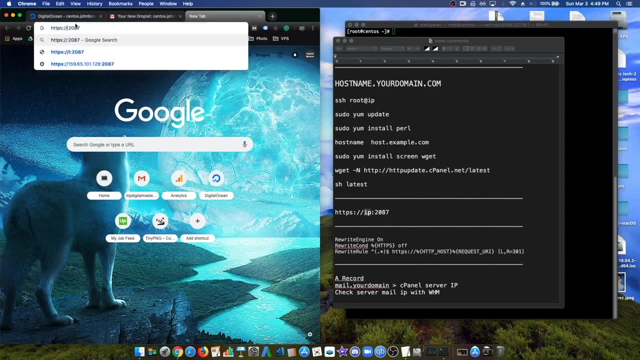 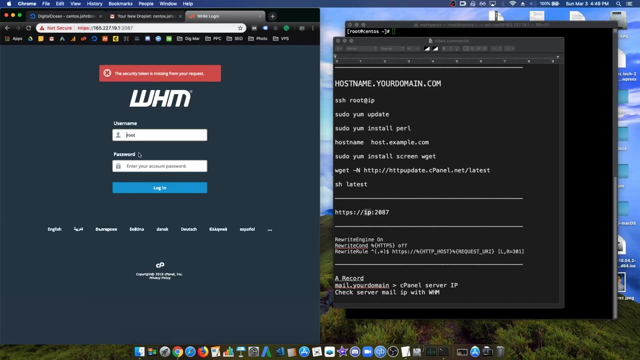 and paste this inside and we're just going to copy our own uh ip right here. so there's a nice clipboard option that we can just choose and just head on, head on over to the link. so it might give you this like no http ps, but it's totally safe. you can just still log in. so just log in and you might. 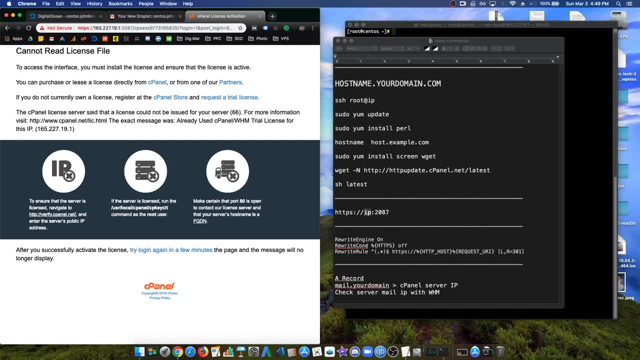 get this if you've done this before, for for me i already already have a server, so it's obviously going to tell me like, after purchase a cpanel license, but for you it might, just it might- give you like the interface and it's going to give you like all these, uh, all like this, like um, it's gonna just give you. 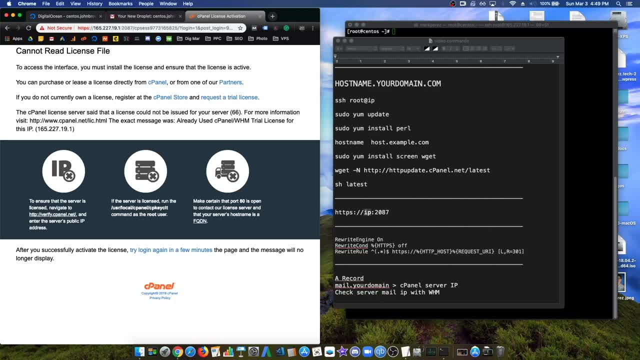 like a setup. it's gonna ask you for certain settings and stuff and most of the time you just wanna, you just wanna click on the default options. so, um, if you, if you need to buy a c light, a c license, uh, um, license, all you, um, you would just go to. 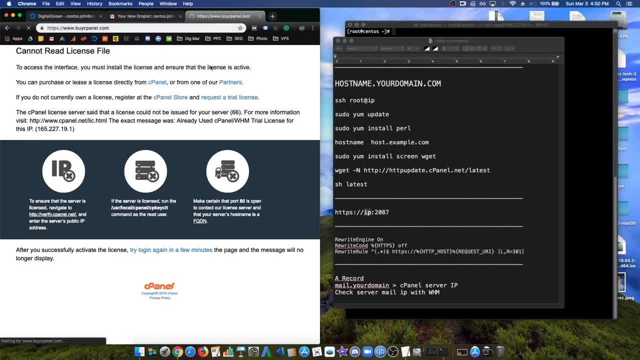 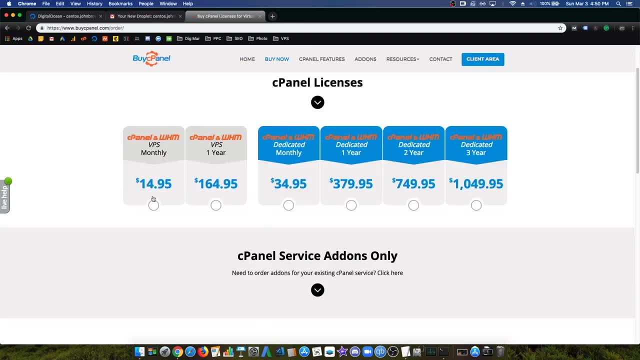 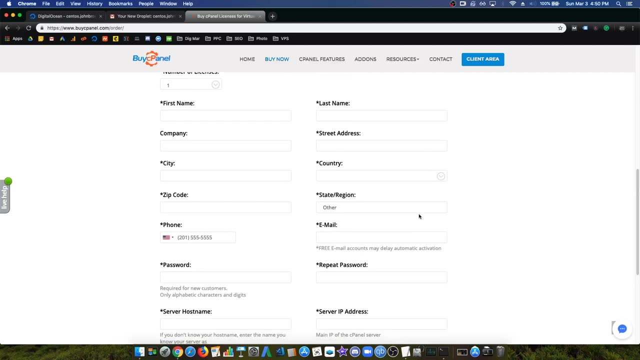 to buycpanelcom. so head on over to this website and just click on buy now. and you want to click on vps monthly and down here you just want to fill up the information and you only need one set of licenses. so after you get your license afterwards, just log right back in. 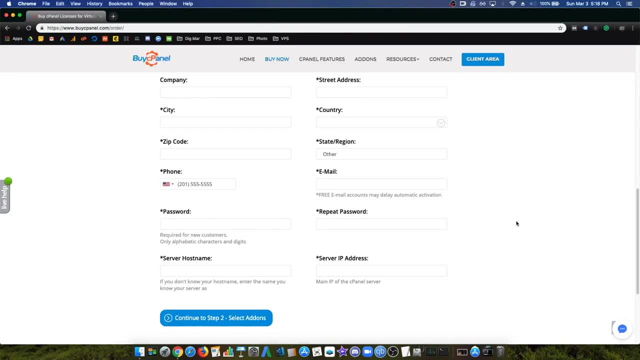 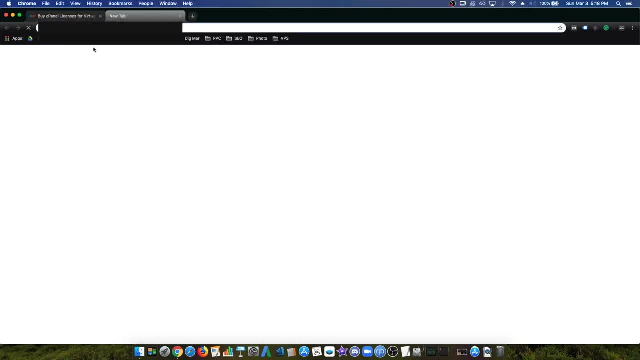 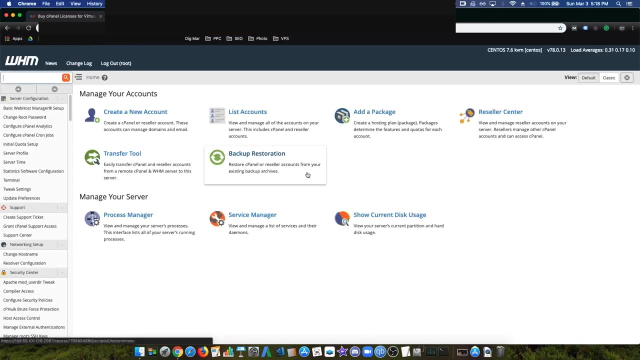 and you should be able to start using cpan. all right, so once you purchase panel account now you actually want to log in into cpanel, so, um, so go back to the link that you had before and just log in as root type in your password. all right, cool, so you have um. now you're. 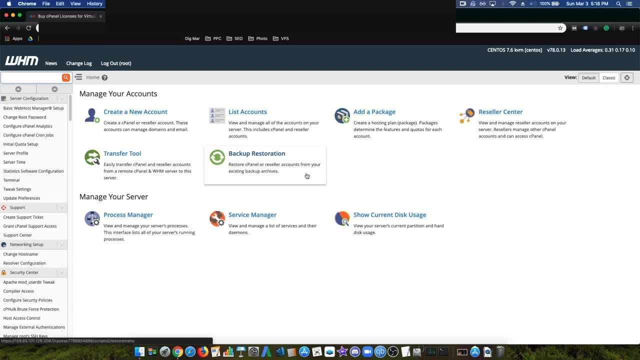 introduced to the whm interface. i'm going to be honest with you. i actually did not use all these settings. i only used like five or four, or probably even less, because, uh, honestly, we're just, you're just managing websites, so you don't really need all this information and as of now, we just we're. 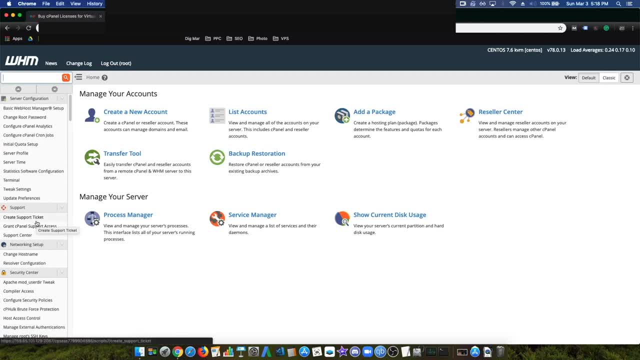 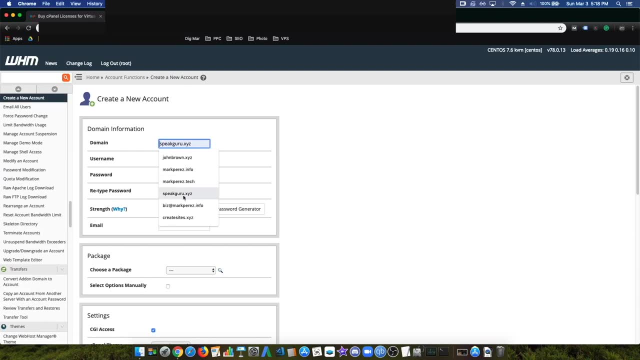 just gonna create the account for our domain. so just go go on over to list accounts and click on create new account and just type in your information. so, uh, for the domain it was john brown, type in your password. email package is default and the rest is technical jargon, so you don't. 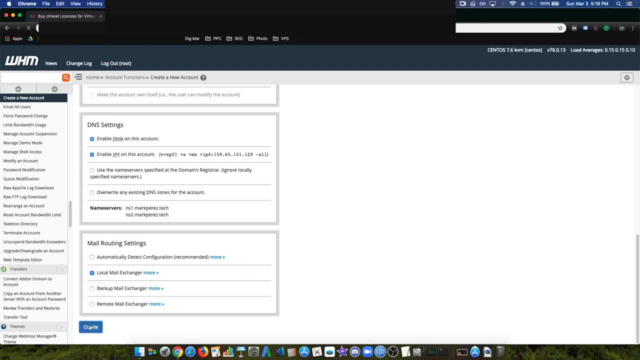 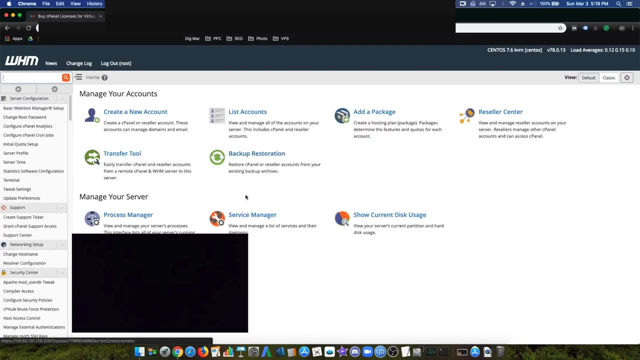 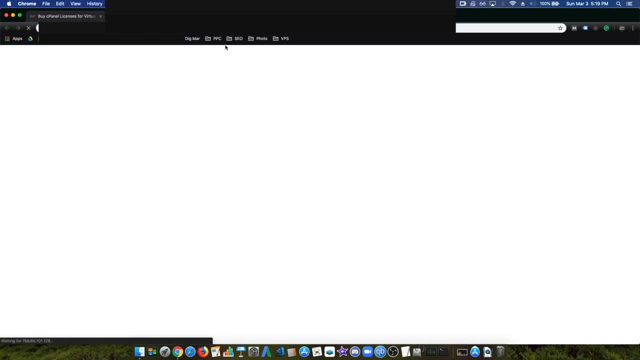 really have to do this. do any of this and just click on create account- awesome, so our account is created. so head on over to the top left corner and click on whm and list your accounts in there, and it should be your account right there, created. so now you want to click on cpanel? cool, so our cpanel is created. so 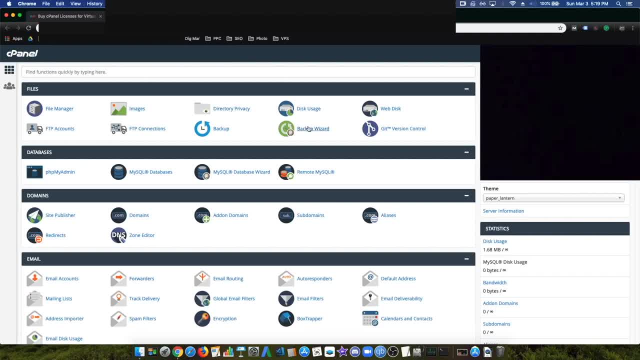 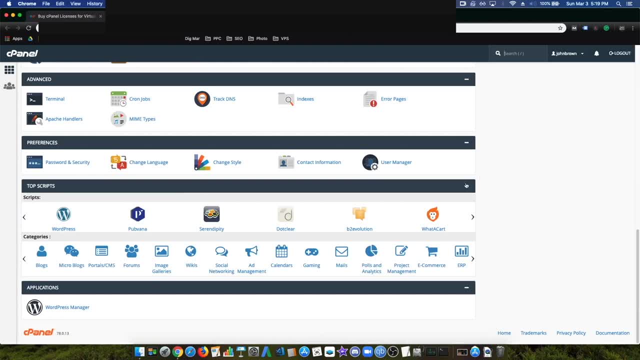 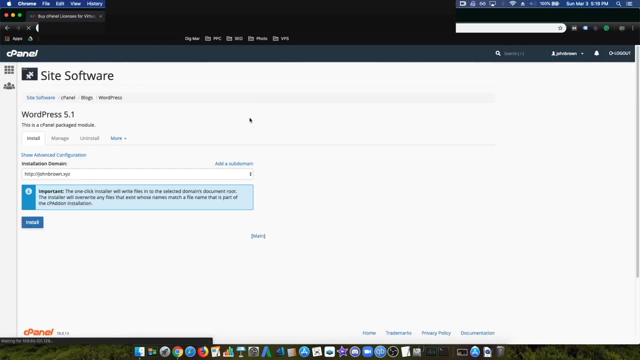 again, this is all information you don't really need. uh, you'll learn this over time, or what you need, so you just want to now. we're just going to install wordpress, so just scroll down and click on wordpress manager. we're going to install the website, so create a new website, and we're going to click on show. 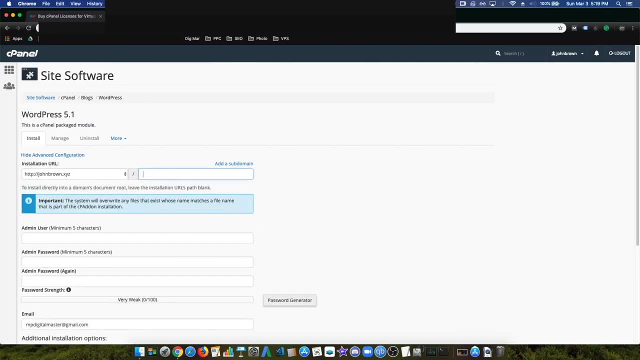 advanced configuration and we're going to delete this because it actually messes up our permalink. so we don't really want to do that and for our user, we're going to type in just the same thing, john brown, and put in your password. yeah, and that's it. so just click on install. 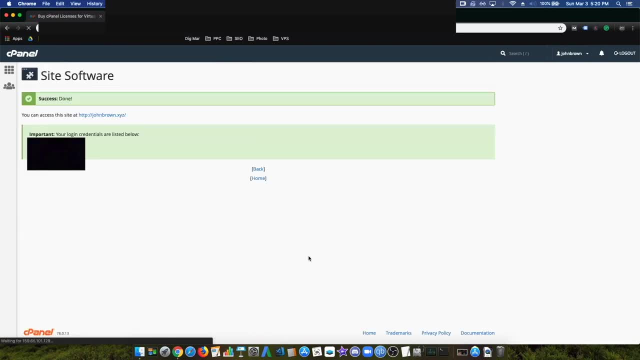 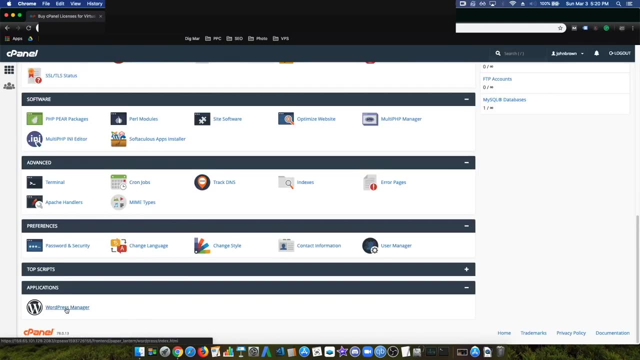 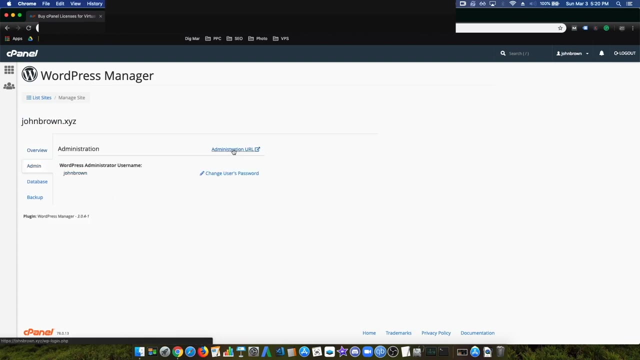 cool, so we installed our url. so just click on home and just scroll all the way down and click on the manager again and click on manage on your domain and click on the admin tab and click on the admin url. cool, so let's just log in. john brown. 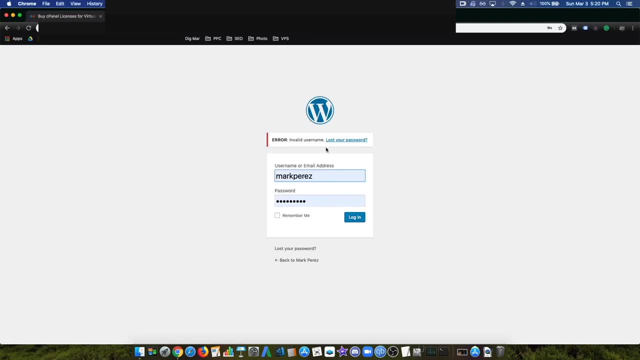 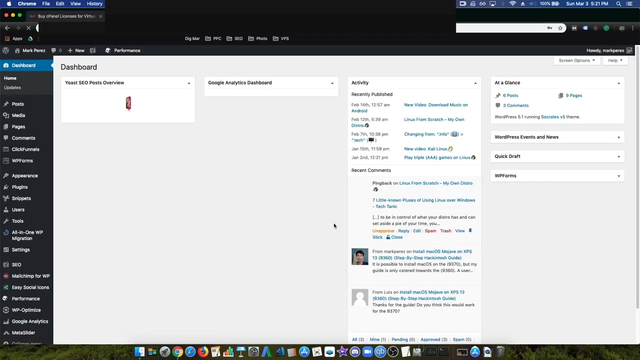 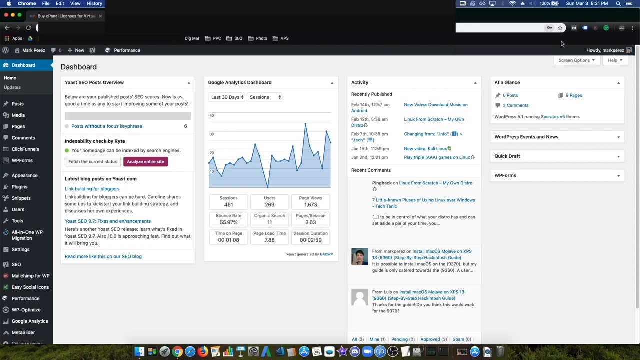 let's see, john brown, that should be right. yeah, let me actually type in the um. yeah, i guess the eml does work better. so here, um cool, so we installed wordpress. um, so, here, um cool, so we installed wordpress. And if you use WordPress before you know, you know how to set up the website, right. 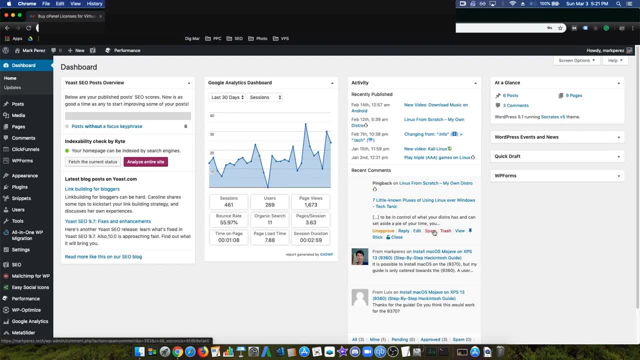 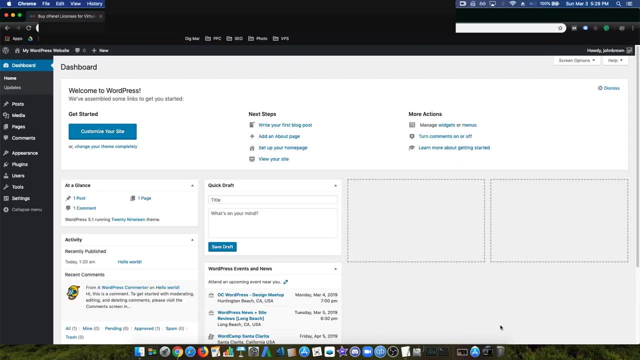 But if this is your first time, I'll show you, like a brief introduction of how to make webpages, how to create blog posts and stuff. So, yeah, All right. So, some of you guys, if this is your first time creating a website, you might not have HTTPS enabled. 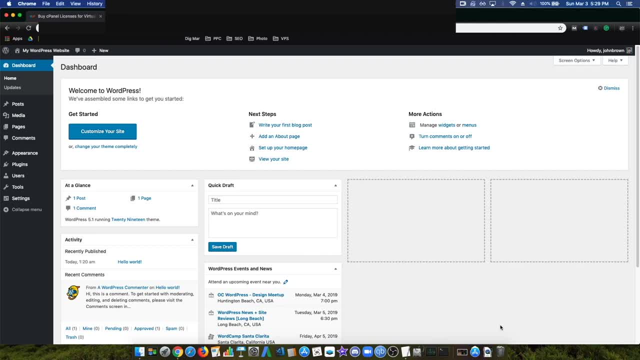 And it's because you actually haven't configured it And you actually don't have to buy like all these like certificates, SSL certificates- that might cost you money And you have to pay for every month or every year, which is actually pretty annoying. 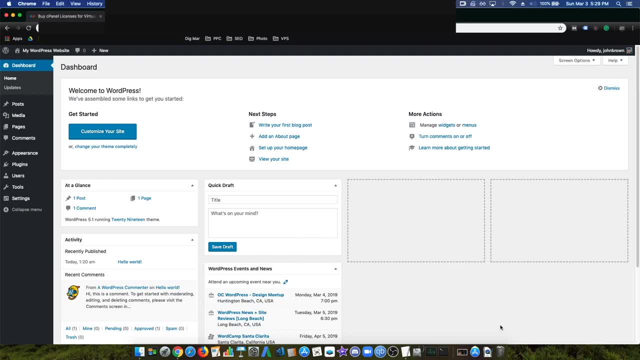 But for us, if we're using a VPS, we can actually get HTTPS for free, which is totally cool. So, in order to do that, it's a bit technical to set up, But don't worry, I'll do this with you. 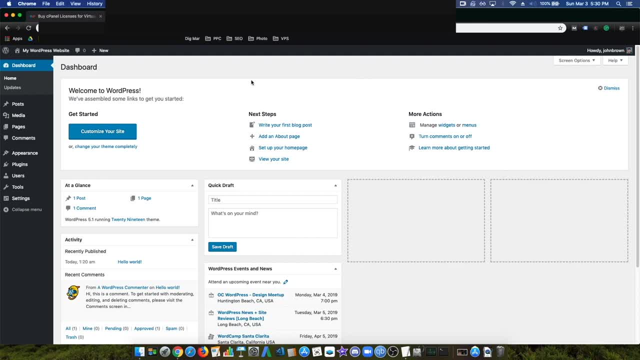 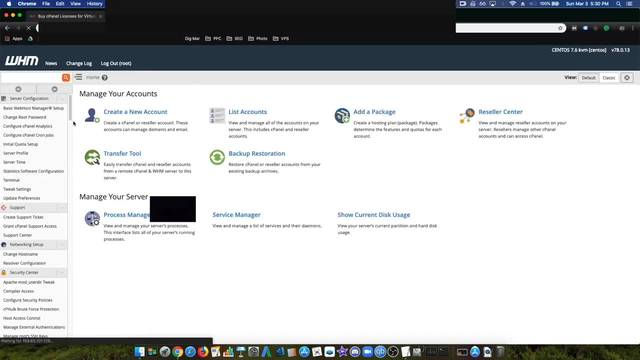 I'll show you how easy it is. So first thing you have to do is go to your – not cpanel. Go to WHM and just go to the main page And you want to type in auto SSL. Click it right there. 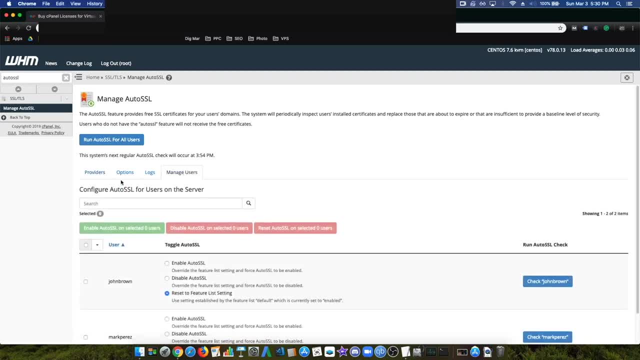 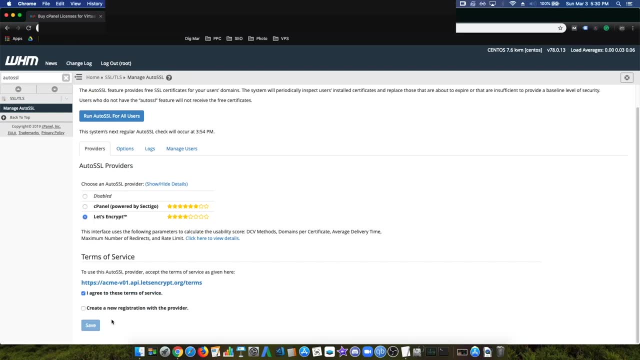 And click on manage users. Actually, before you guys do that, go to options and make sure let's encrypt is enabled And you want to agree on the terms and conditions And you want to click on save. Let me check if there's anything on the options. 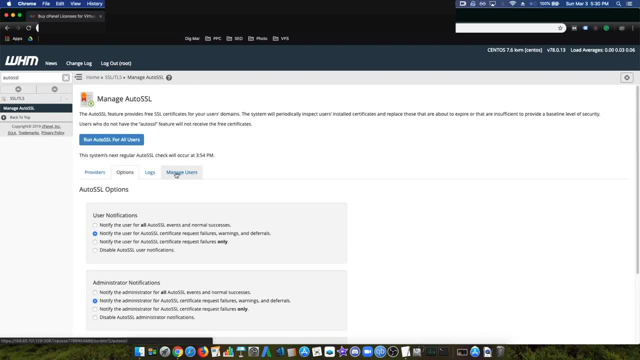 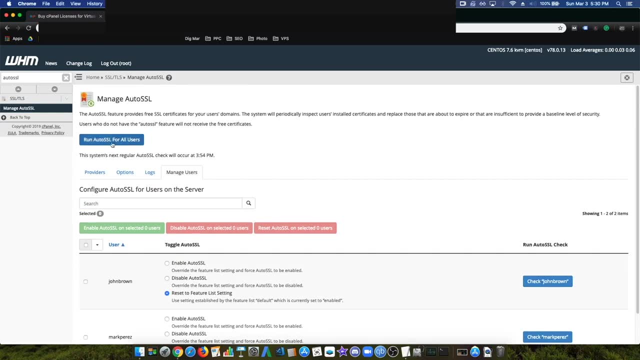 Yeah, I don't think you have to really configure it right here And for manage users, make sure you have enabled auto SSL And afterwards now we click on run auto SSL for all users. So now we actually have HTTPS, But we're not done quite yet, because we actually now have to tell the links to actually go to HTTPS, which is a bit complicated. 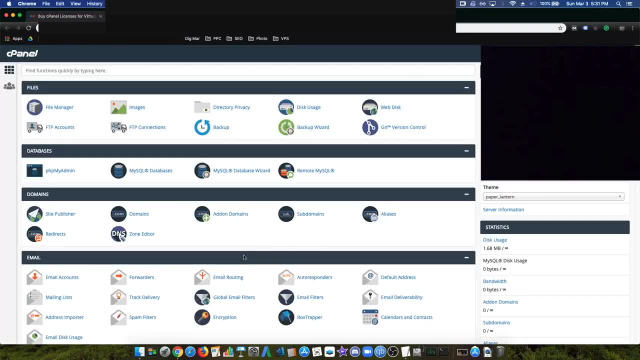 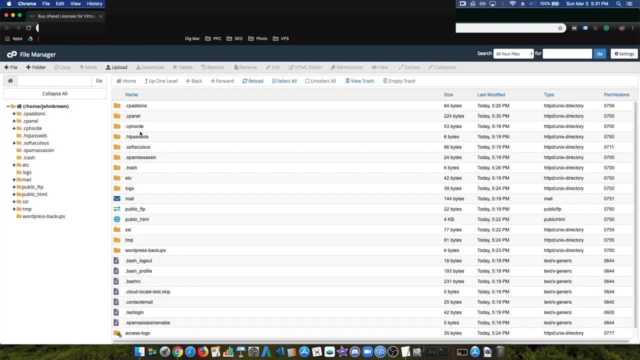 But don't worry. So now you want to go back to your cpanel account for your domain. So now you want – and then afterwards you want to click on the file manager, And this might be a bit complicated, But don't worry. 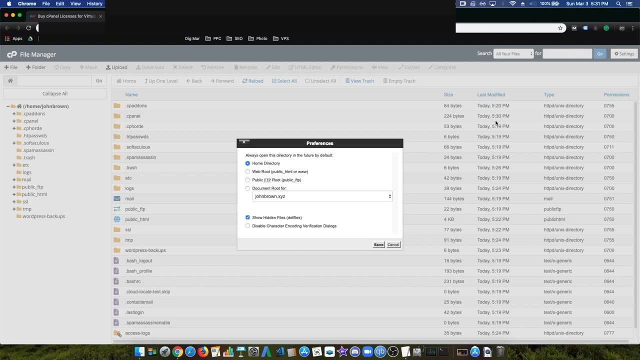 This won't be too bad. So you want to click on settings And make sure you have show hidden files, So we actually, like, can edit a hidden file inside our computer. So afterwards just click on save Cool, And then on the left-hand sidebar you want to click on public HTML.